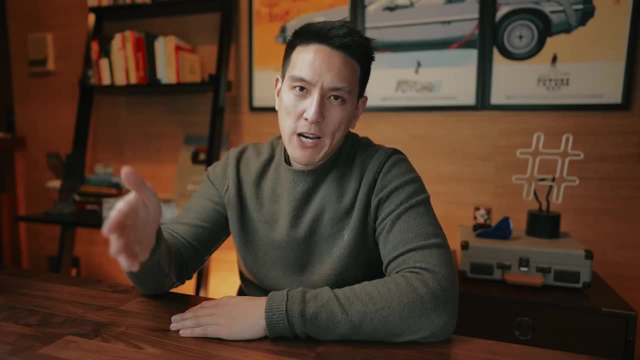 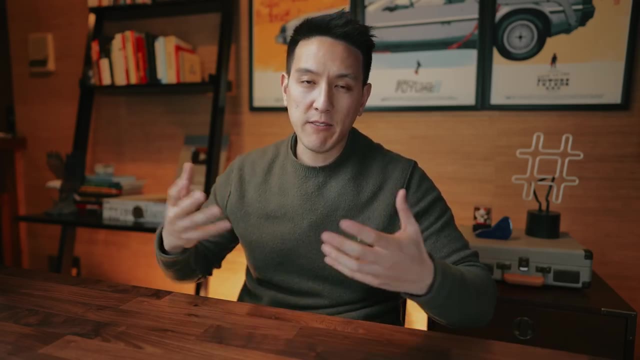 want to save money. it can help you save money as well. The first reason why Chinese people like to save money is the meaning of money and what it means to them. So as kids, you're taught from a very early age that saving money is honorable Kids. 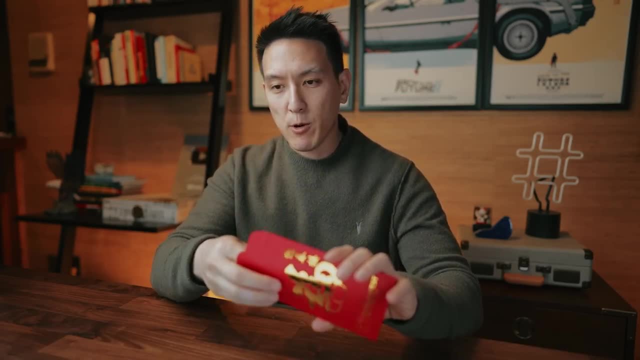 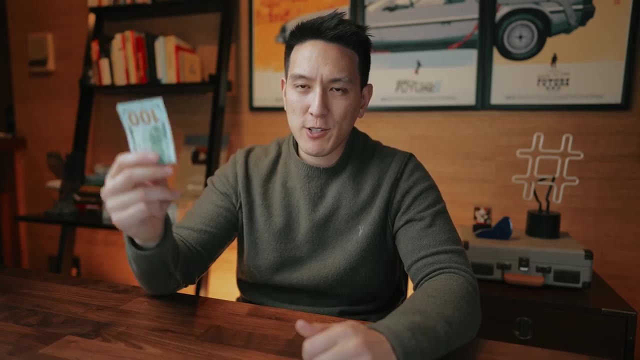 will often get money in these red envelopes for New Year's and birthdays, and they are often encouraged by their parents to save it. This money is referred to as lucky money. Now, money is so important to the Chinese that they even have a phrase during the holidays and New Year's that 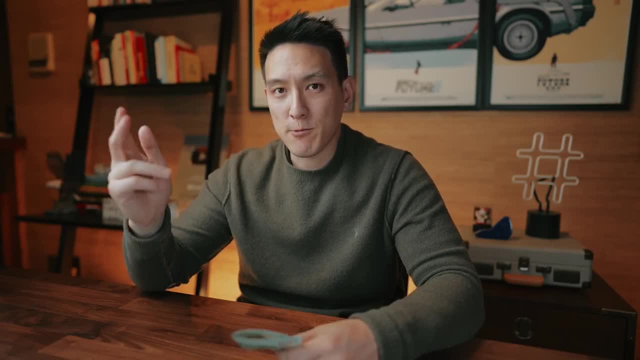 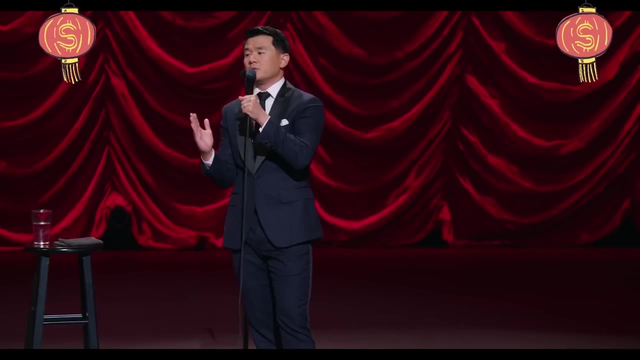 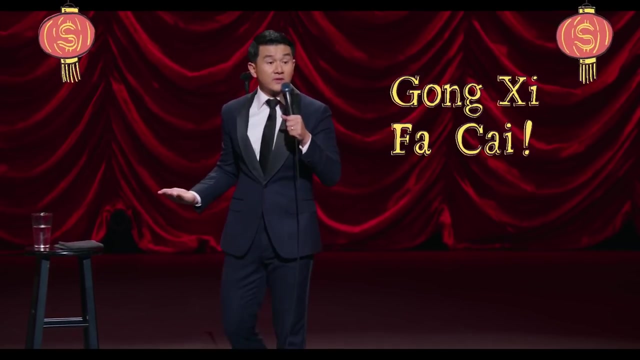 they say: Instead of Happy New Year, they say something else. Let's listen to Ronnie Chang, the comedian, explain it better than I can. The biggest holiday for Chinese people, Chinese New Year. When we see each other during Chinese New Year, the way we greet each other is, we say in Cantonese: I'm sure you've heard that at least. 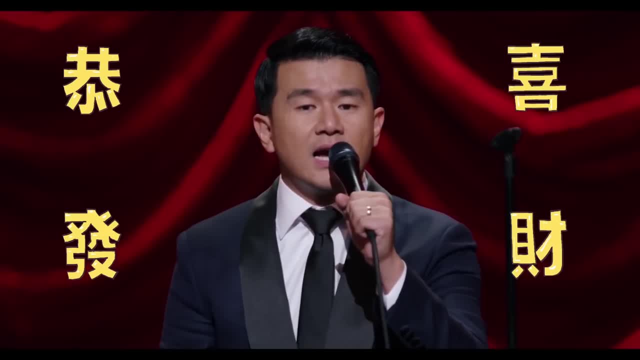 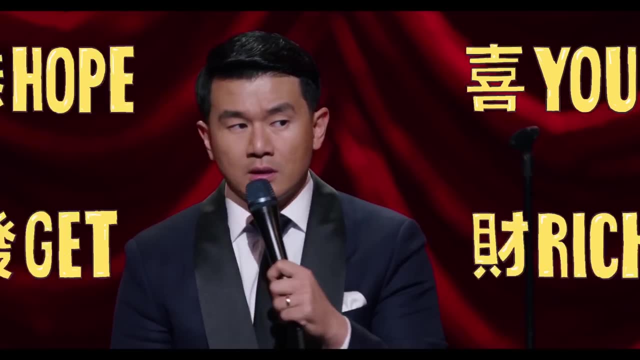 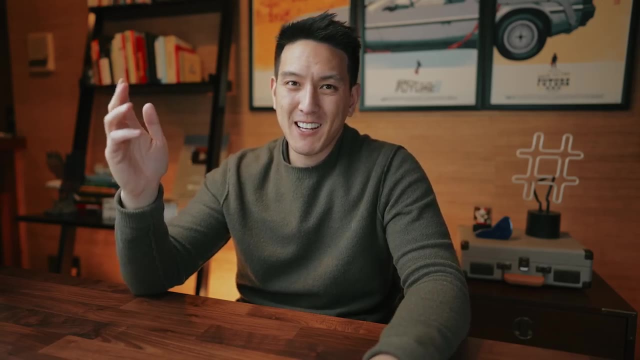 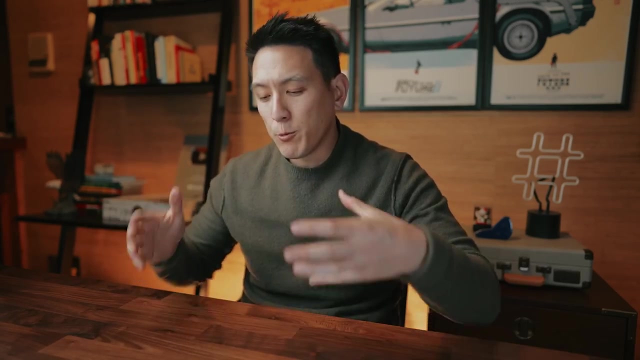 prayerfully right means hope you get rich. That's not Happy New Year. That's pretty funny because it's also true. You can also see the importance of money in the way that people in Chinese society treat other people with a lot of money, People with a lot of money. 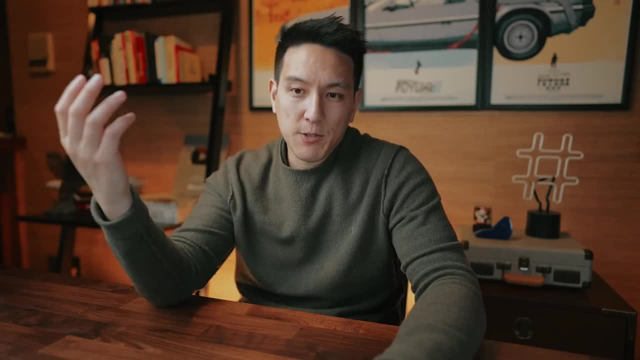 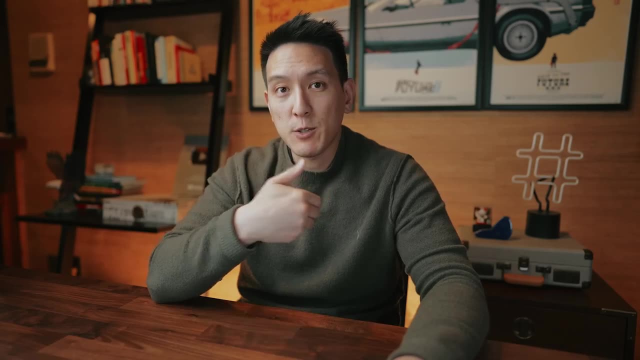 in Chinese culture are deemed successful in many people's eyes, and so it's often viewed as a good thing to have a lot of money. Now, being successful also has its other perks in China, and that actually brings me to my next point, which is demographics. Up until 2016,, China actually had 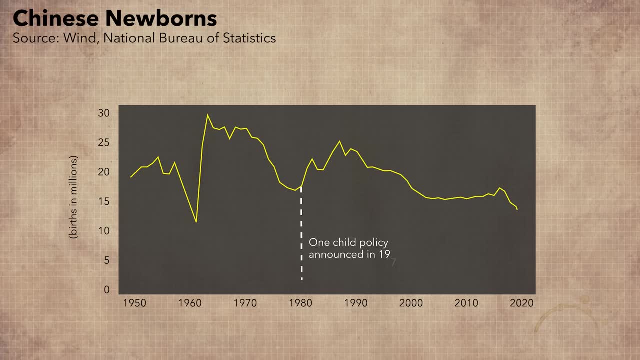 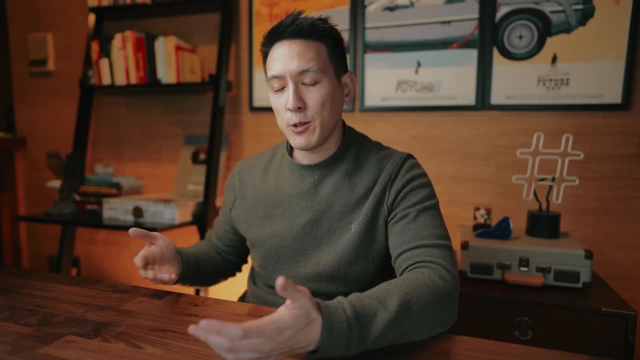 a one-child policy that was implemented in the late 70s and early 80s to kind of stem overpopulation, and that means each family could have one child. Now, if you had more than one child you would just be slapped with a fine and in addition, if you didn't pay that fine, 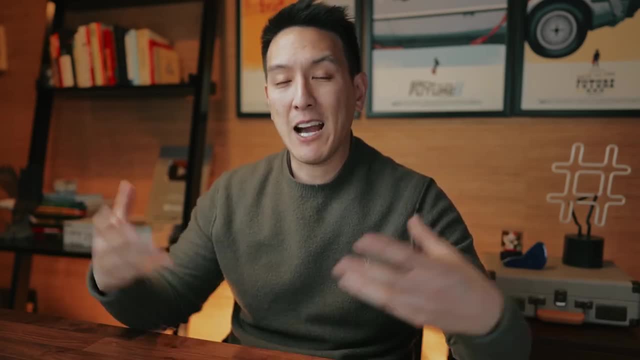 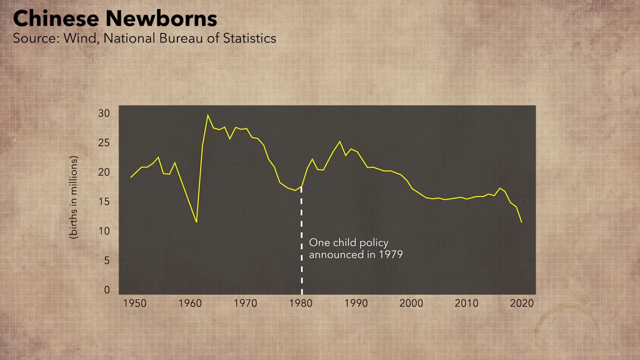 your household would not be able to register your second child's name in the household system, so your second child would not be eligible for healthcare services and other services like education. So naturally, this one-child policy created a sharp decline in newborns, as you can. 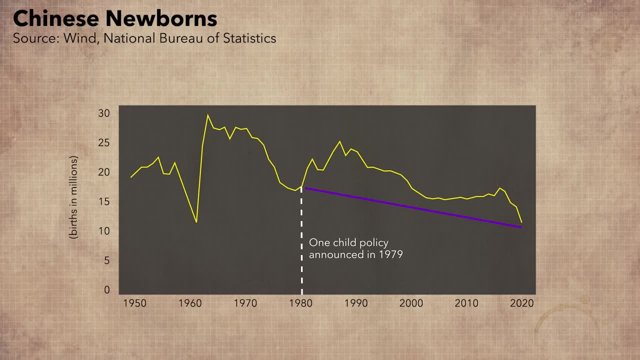 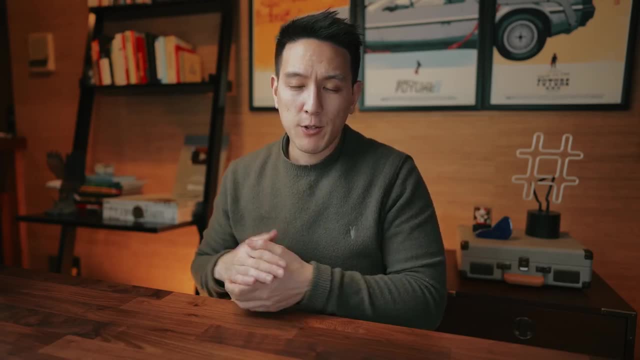 see by this graph, but also in sex-selective abortions In China, it's usually much more important to have a boy than a girl. So in China it's usually much more important to have a boy than a girl, because the boy usually inherits the family name as well as the property. So what you 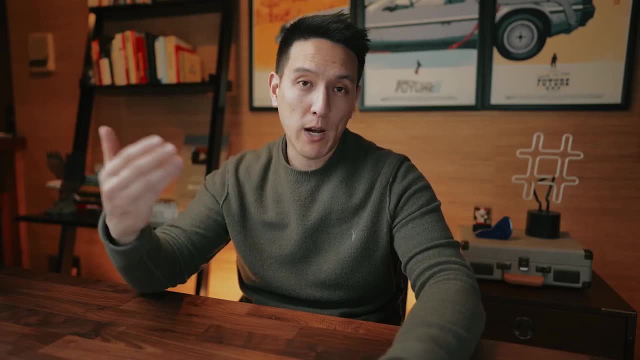 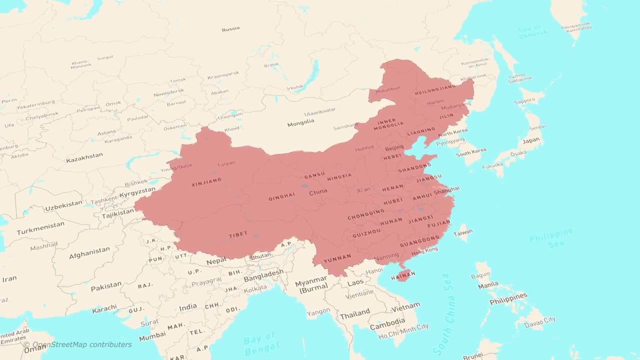 had was a lot of people kind of using contraception in a way that they would avoid female births and try to optimize for male births. And with that contraception actually it skewed the population, having more males than females over time. So at its worst it was 122 males for every 100 females. 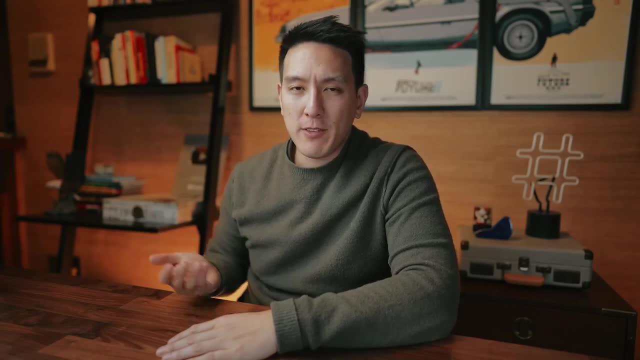 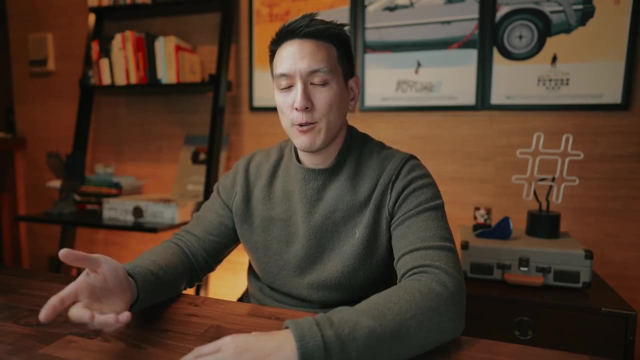 that were born Now. in general terms, if you have more men than women, then you have a supply and demand issue, right? So there's more men chasing the same amount of women. So basically, to stand out as a man in China, you have to be viewed as successful, aka you probably have a lot. of money. The other thing with the one-child policy was that since families were only having one child, they weren't having multiple kids. in the majority of cases, That means that the parents could save more money because they didn't have multiple kids to feed. So you kind of had a double whammy with. 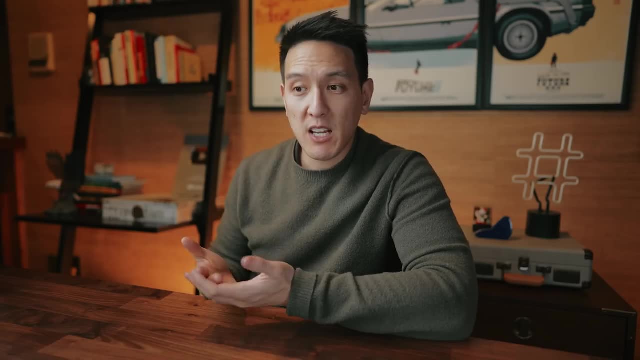 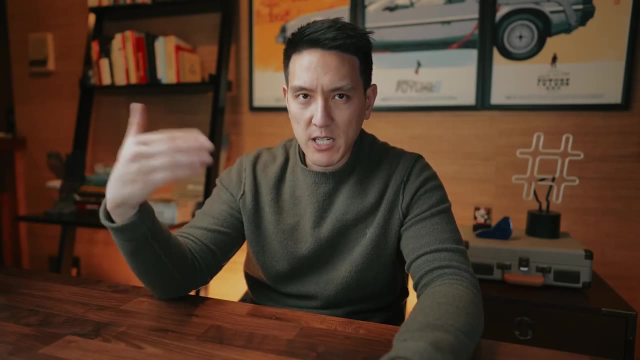 the one-child policy. You had parents not having to spend as much money and then the males trying to save as much money to become desirable. Another reason for saving in China is that there's no 401k, there's no IRA, there's no retirement accounts that Chinese people can. 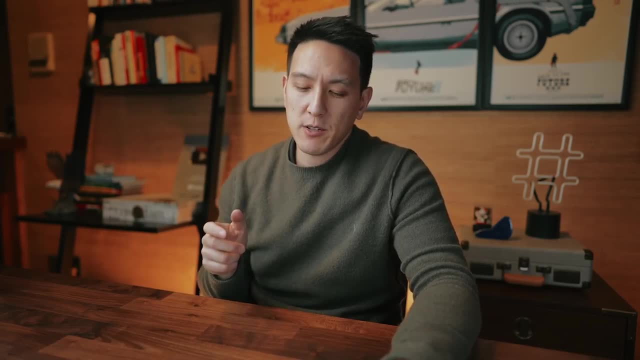 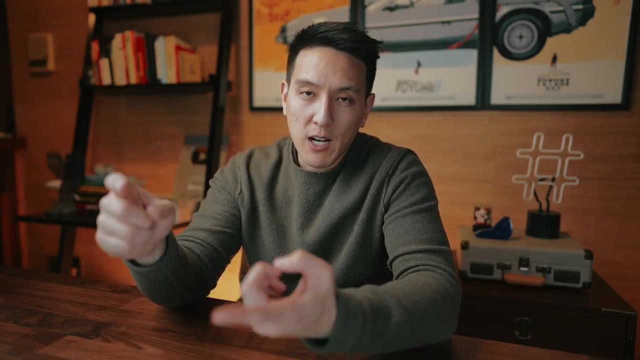 contribute to. Rather, they do have what's called a pension system, but still many people in China are wary that the pension system will still be around when they retire, and so they also worry about the costs of healthcare, education and their own pensions. So these are some of the 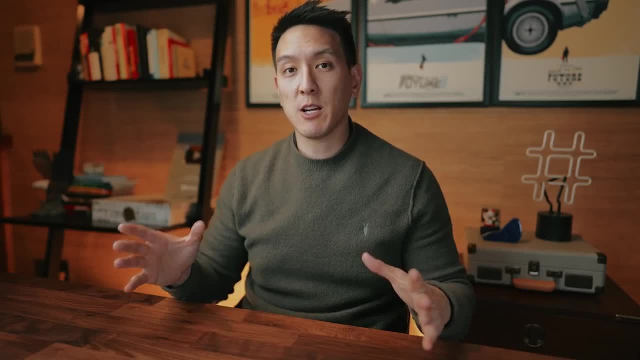 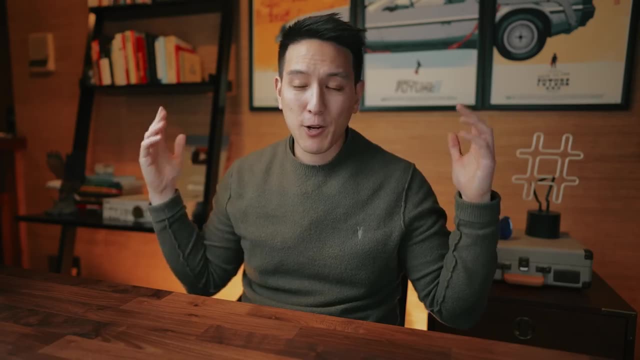 intrinsic reasons as to why Chinese people like to save money. but let's actually talk about the money secret of this video, The main secret as to why Chinese people are brilliant at saving money. it's not anything crazy, It's just that they have every dollar accounted for. In my particular case. 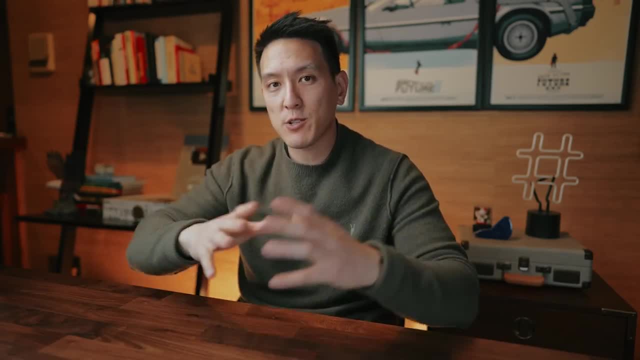 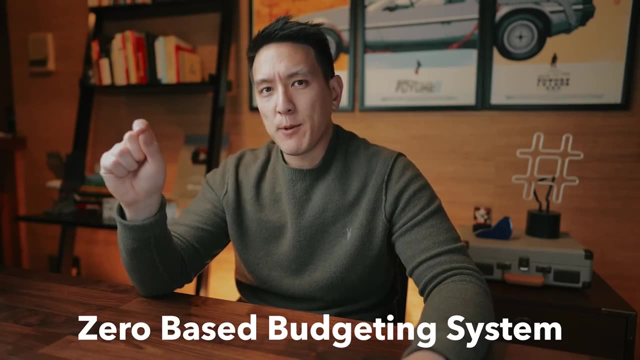 where his money was going at all times. and there is a special budgeting system that can help you with this, and in America and in the Western countries it's called the zero-based budgeting system. The zero-based budgeting system is a method in which you budget where you spend every. 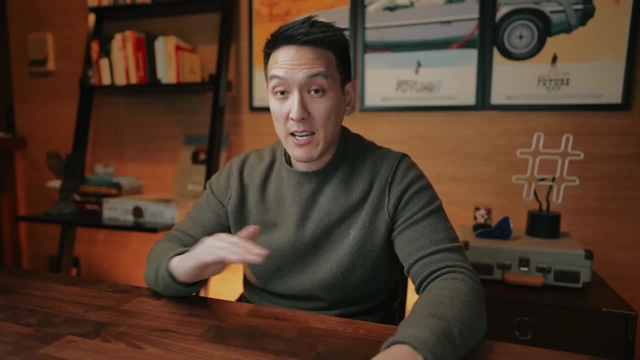 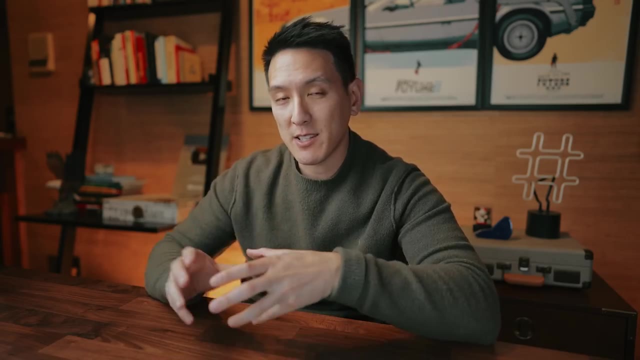 last cent of your monthly income, so that your amount left at the end of every month is equal to zero. So that means your income minus your expenses equals zero at the end of the month. Now, expenses in this case also includes savings, investments, paying off debt, etc. Let's pretend. 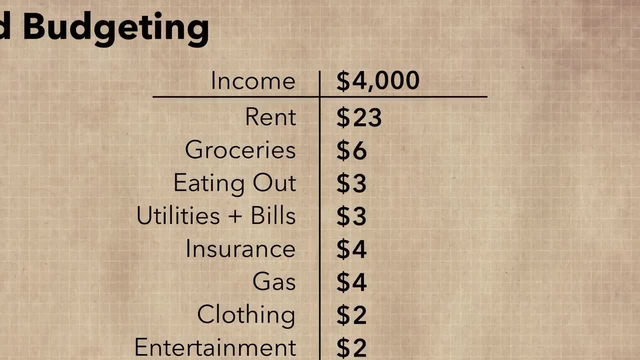 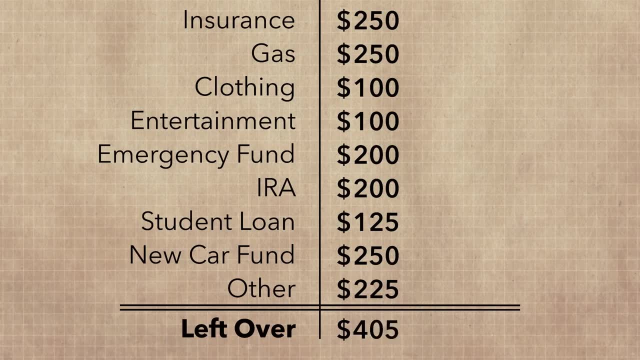 you make $4,000 a month. A zero-based budget might look like the following: You have your rents, your groceries, your necessities- all listed right here, but then you also have a section for the things that you're saving for Your emergency fund, your IRA, your student loan payments. 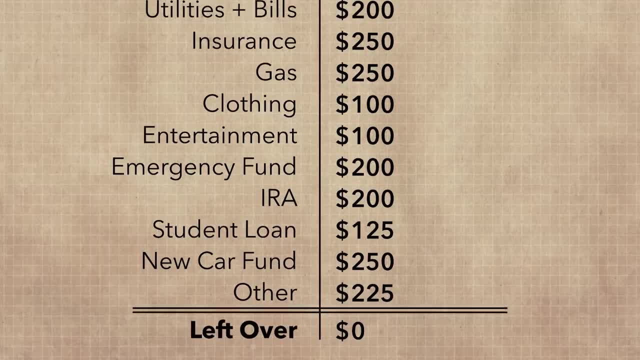 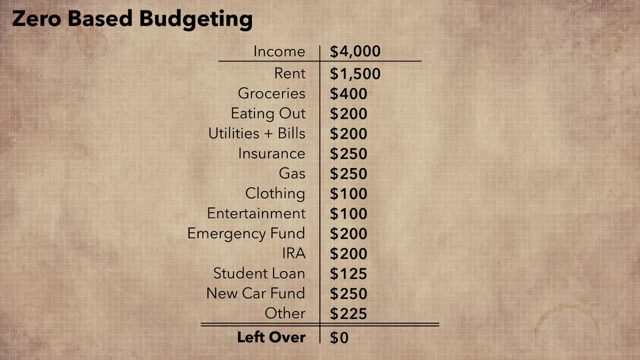 new car fund and then any other savings that you might want to do. You can see, by the time that you get to the end of your budgeting, you are left with zero dollars at the bottom right here. This is essentially the zero-based budgeting system, where all dollars are accounted for. You can. 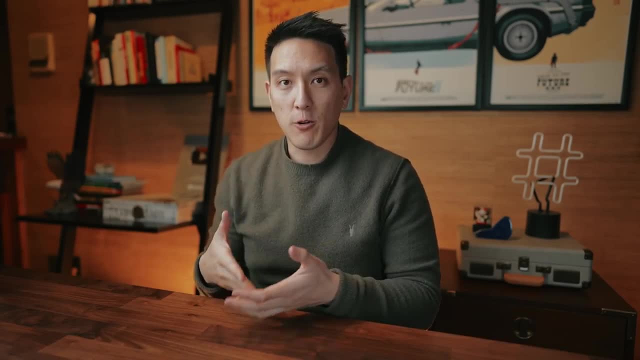 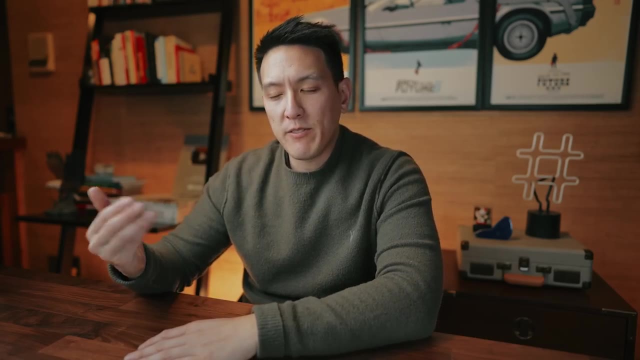 save a lot of money, but it also means that you have to be super honest with your own expenses, And sometimes you might have to do this for three months to get an average of all your variable expenses throughout the three months. If you've watched some of my videos before, you should know. 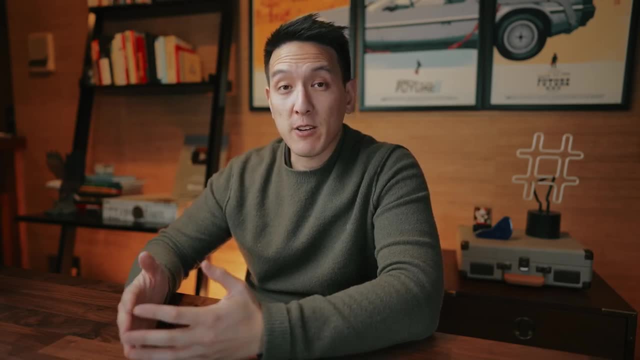 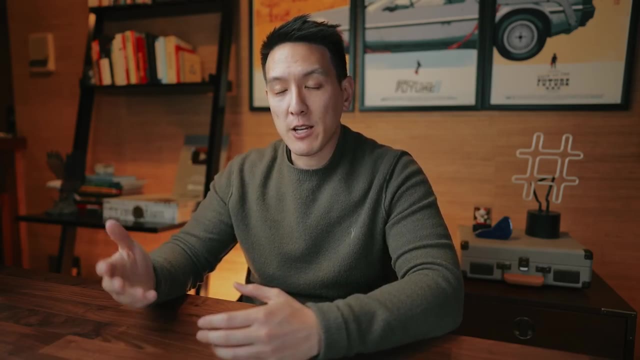 that this budgeting system doesn't exactly tell you how much you should spend for every single category. Rather, it kind of helps you understand your expenses as a whole, including your fixed expenses, and then you can kind of categorize your expenses and allocate your budget from there. 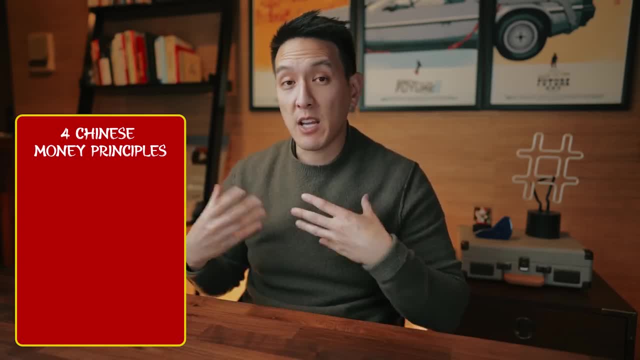 All right. there are four main factors that the Chinese prioritize to help them save a lot of money that I want to tell you about. The first one is the cost of living. The second one is the cost of. Before we do that, though, make sure to drop this video a like, and if you enjoy economics and 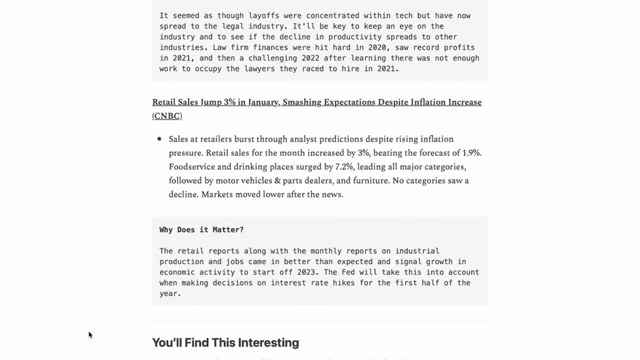 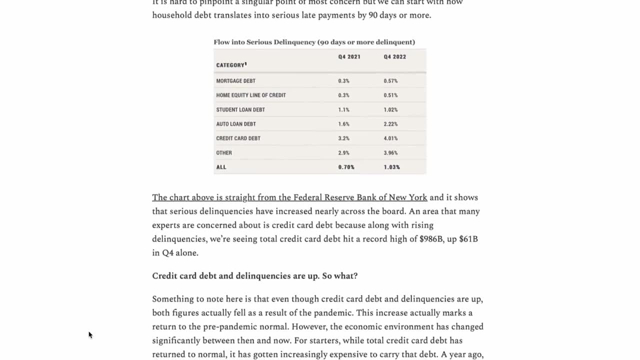 business content. I want you to check out my free newsletter called Hump Days That comes out twice a week on Wednesdays and Sundays. It's completely free to sign up and I will link it down below and I hope to see you guys in the newsletter as well. All right, so the first of the four. 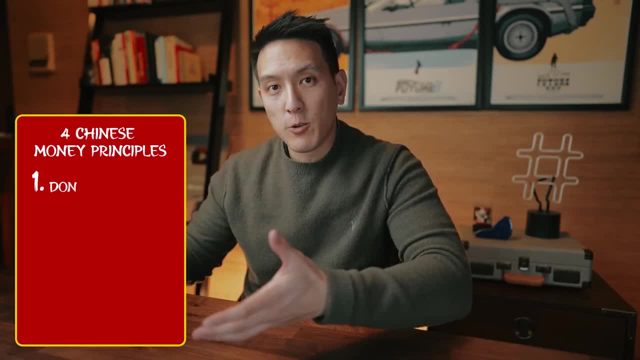 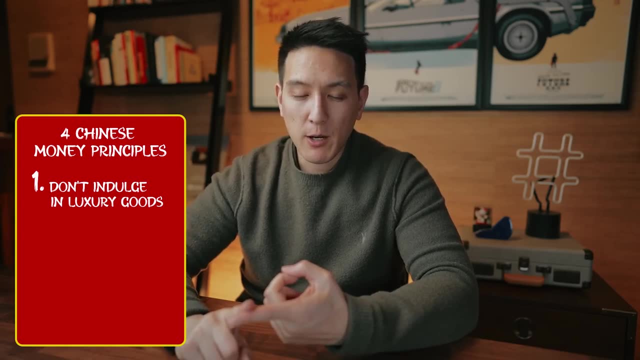 main factors that the Chinese do to help them save money is that they don't indulge in luxury goods or goods that are just there as status symbols. The majority of Chinese people want to stay humble, and they also want to fly under the radar, so they usually stay away from the 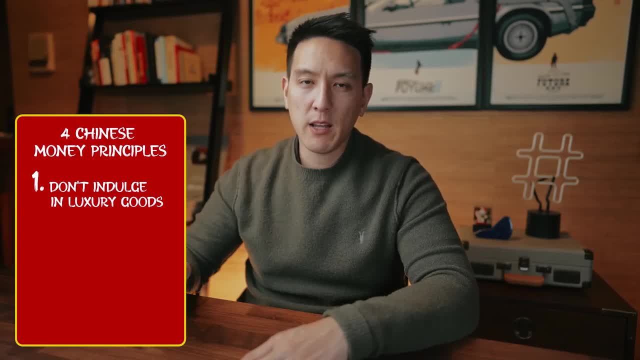 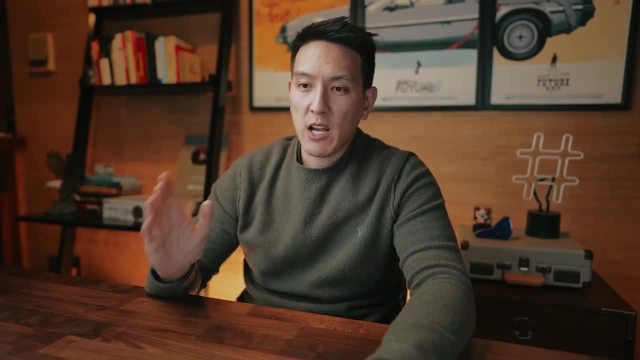 luxury products. Number two: when the Chinese earn money, they usually like to live off a very small percentage of their income. Now, my dad grew up with very little money as a child in Shanghai. There were some days that he could not even afford food and he would go to sleep hungry. 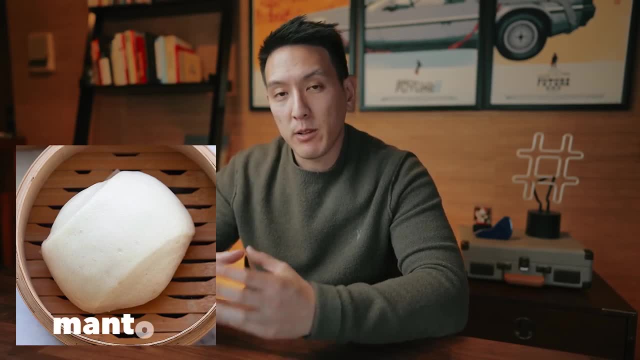 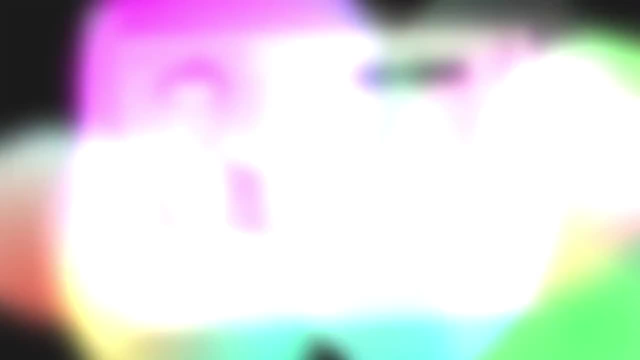 When he was able to afford food. all he could really buy at the time was a plain pastry called a manto, and a manto is a tasteless kind of white bun that you can buy for very cheap. Because of this tough childhood when my dad started his career, whenever he earned, let's say, $10,. 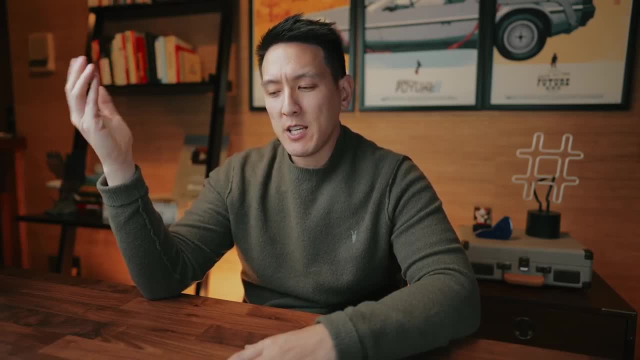 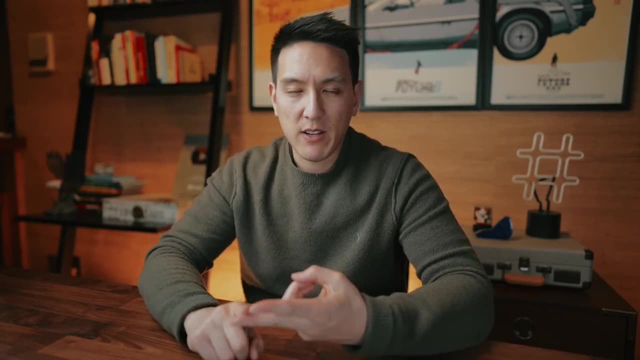 he tried to live off of one single dollar. Now, in reality, was he able to live off of $1 for every $10 that he earned? Not really. There were going to be times that he had to spend six, seven, eight. 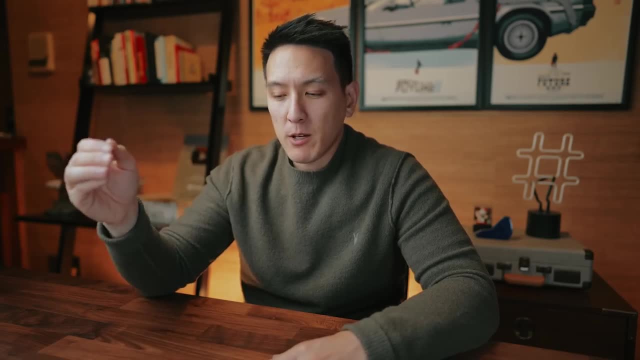 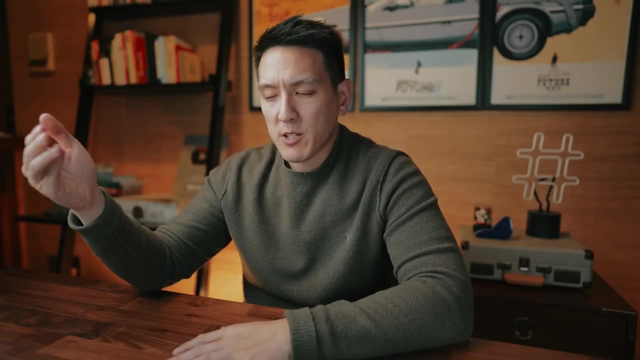 or nine out of those $10 just to make ends meet. For him, though, saving money wasn't a way to build wealth. It was actually a way to ensure that he never had to sleep hungry again. So this simple principle of trying to save as much money as you can and live off of little as 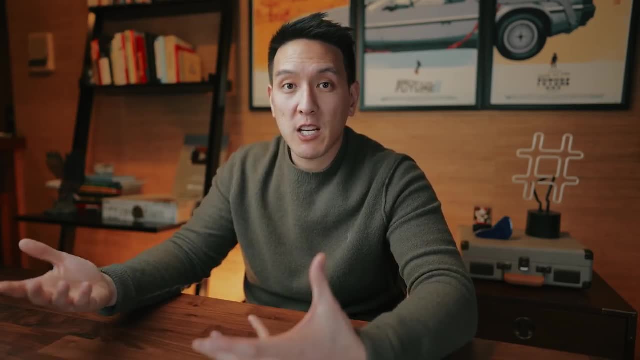 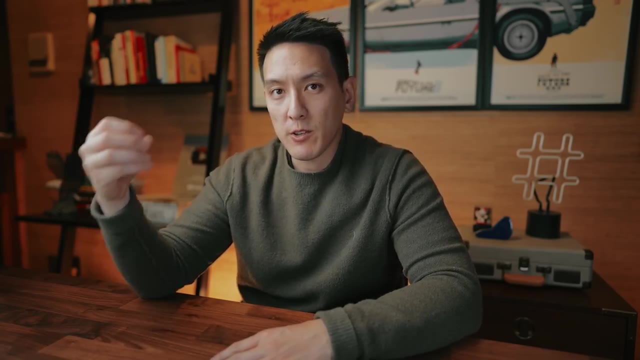 possible really stuck with me, and it's one of the main factors that I think many other Chinese stopped as well. Now, this is a good rule if you're trying to build wealth, but please understand that this type of rule will create what's called a scarcity mindset about money. 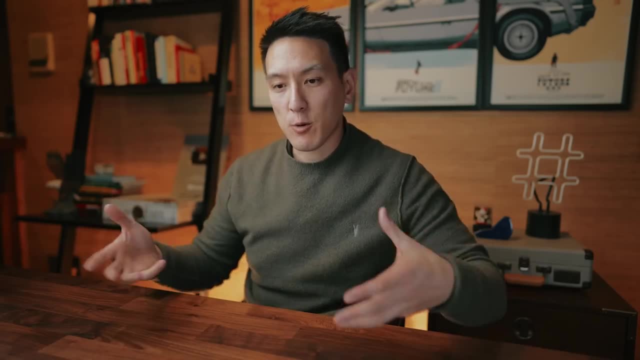 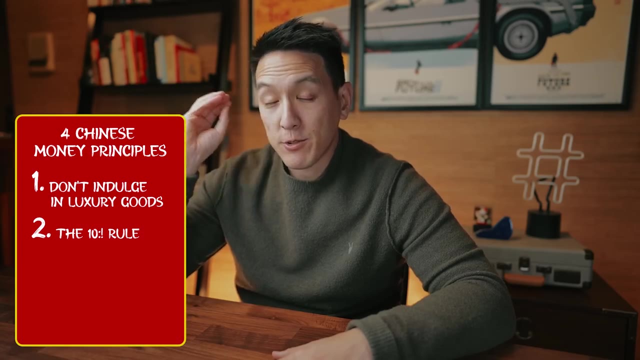 and so you kind of have to acknowledge that psychologically that as you earn more money you can kind of switch your mindset into more of an abundance mindset later on. The third factor that the Chinese employ to save a lot of money is that they really focus. 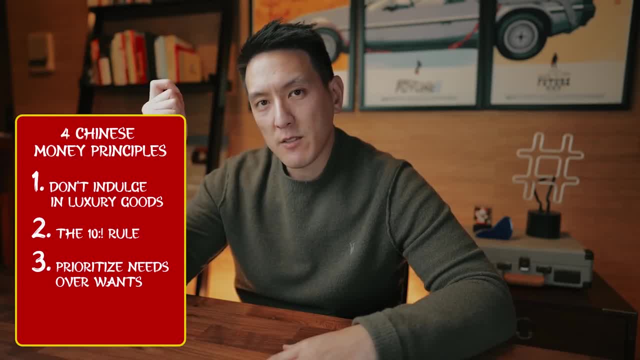 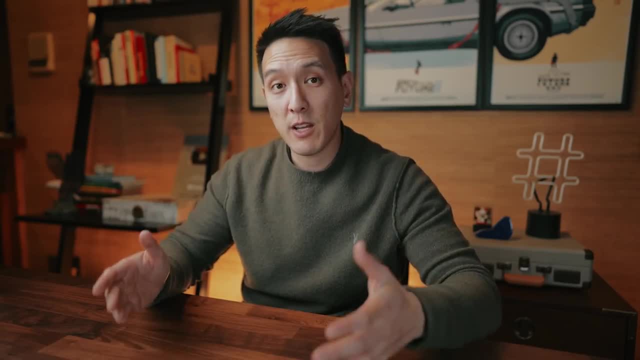 on their needs versus their wants. So another wise lesson from them is that if you need something and you have to actually spend money on something you need, then go ahead and spend money, especially if it pertains to your health. So if you're debating between a flimsy desk chair, 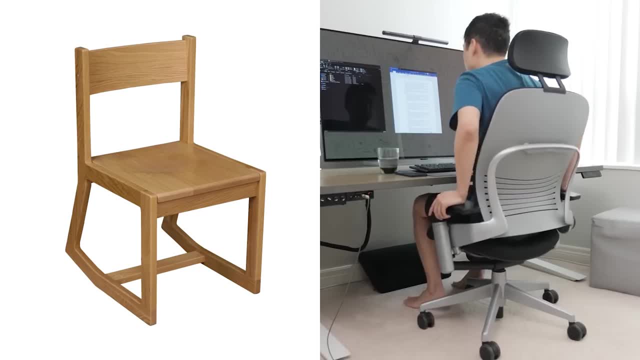 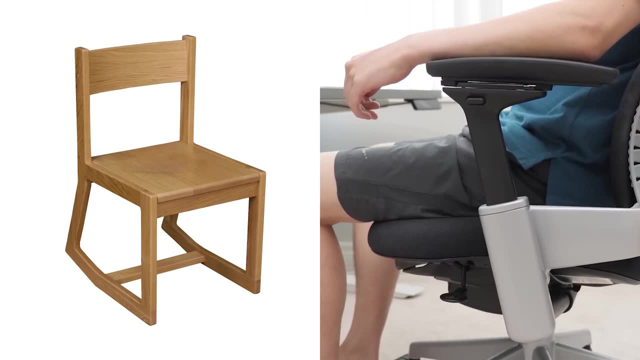 or an ergonomic chair that might be able to make you more comfortable and stay healthier throughout the day. you might wanna opt for that ergonomic chair. I would classify the ergonomic chair as a need within reason. Of course you don't wanna take this logic. 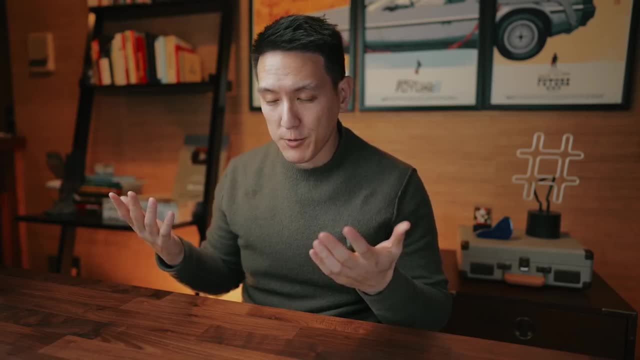 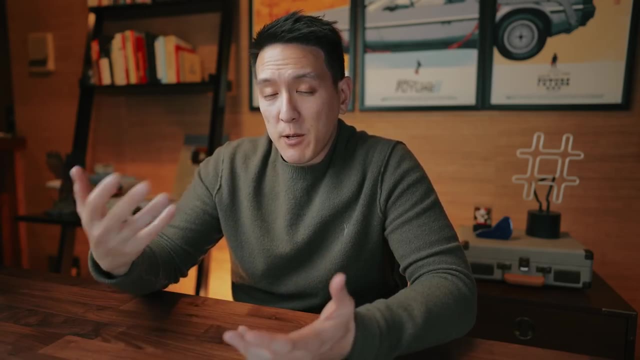 to the most extreme. For example, everyone needs clothes, but that doesn't mean you need to go buy Gucci clothes just because they are better, because it's a need. So here the idea is to be reasonable with your spending and make smart choices. 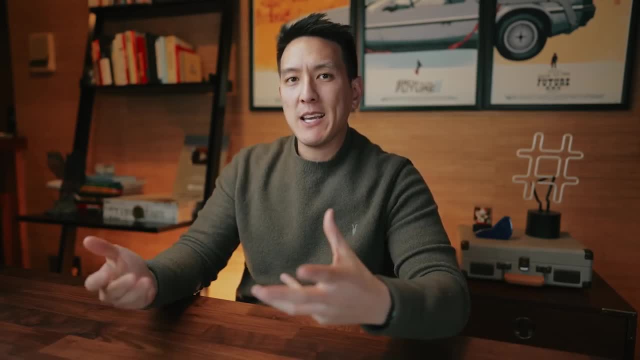 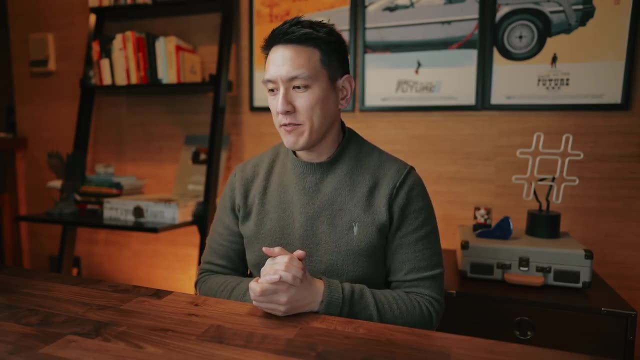 and save where you can. Now, when it comes to wants, you can still buy something that you want, but make sure that you're gonna get really good value out of that. So what do I mean by that? Let's say you buy a $350 fancy wallet. 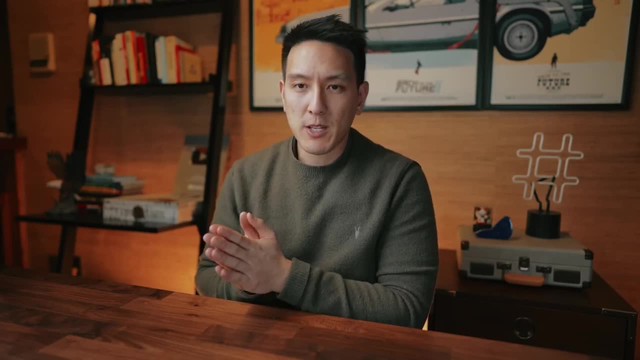 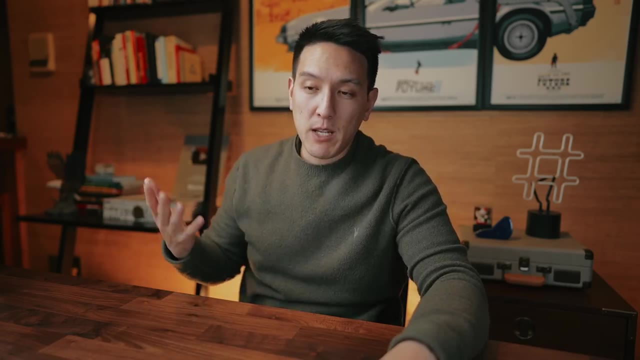 Like, let's say you just really wanted this. Well, you wanna make sure that you can use that wallet for a very long time so that it amortizes the cost of your use. Could you use that wallet for five years Then that means you would take that $350. 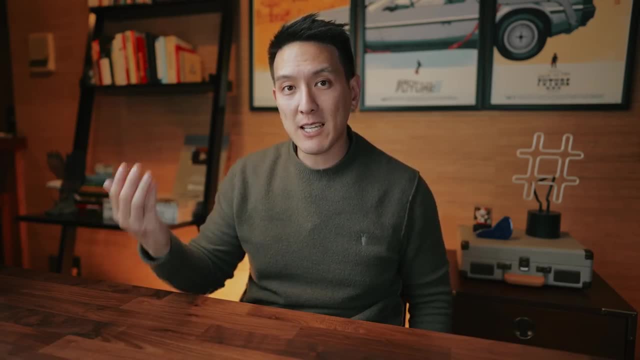 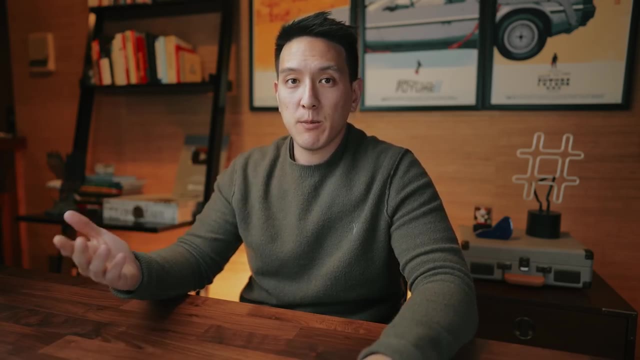 and spread it out over five years of usage, That comes out to less than 20 cents a day. Spending money is inevitable. Everybody will have to spend money at some point, but the lesson here is to be reasonable and frugal with most of your decisions. 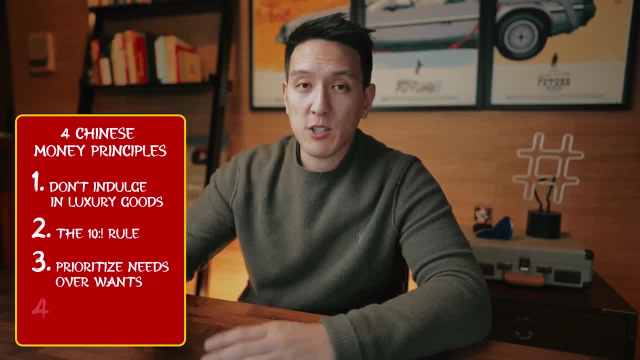 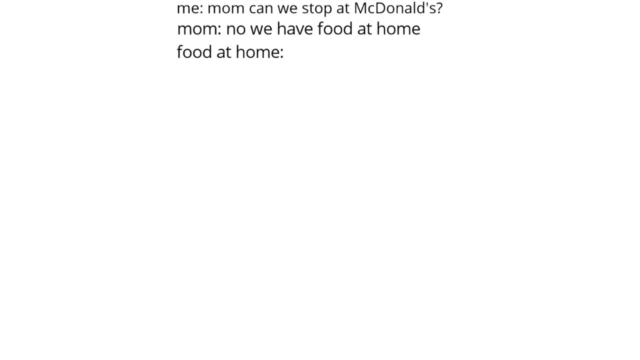 The last factor here is that if you're trying to save money very quickly, the Chinese would advise you to stay at home and eat at home. No, we have food at home. Food at home. I think this one is pretty universal to most cultures.